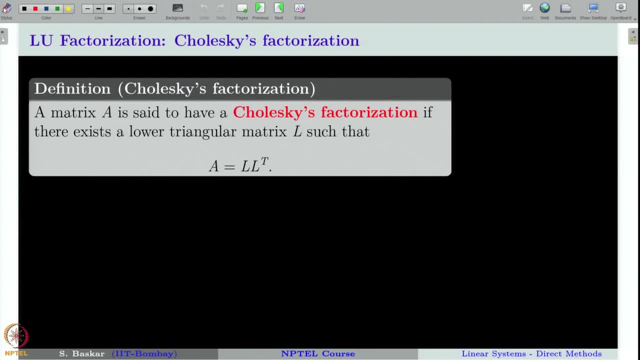 of that you again get L into L transpose. Therefore Cholsky's factorization is possible only for symmetric matrices. Also, we will see that Cholsky's factorization exists if the matrix A is a positive definite matrix. Let us recall from our linear algebra course what is mean by a positive definite. 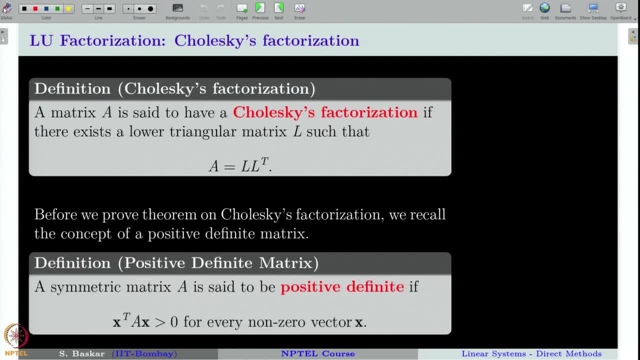 matrix A. symmetric matrix A is said to be positive, definite if x transpose A. x is positive for all non-zero vectors. You can see from this definition that it is not that easy for us to check whether a given symmetric matrix is positive, definite or not. For that you have to take all the non-zero. 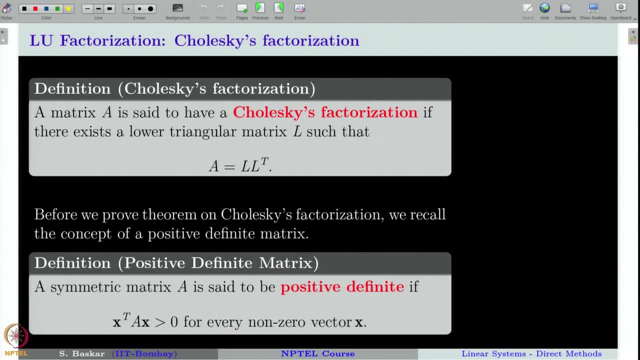 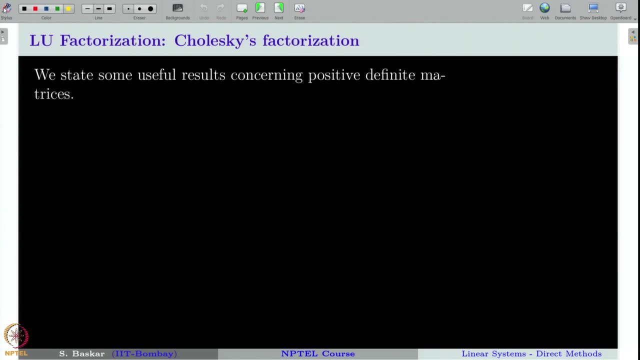 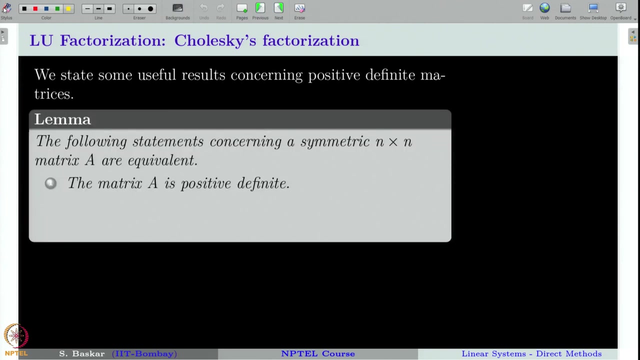 vectors and compute the expression x, transpose A, x and check if it is a positive number. That seems to be very difficult. Therefore we have some equivalent properties which we would have studied in our linear algebra course. Here we will just recall those properties in the form of a lemma, Suppose. 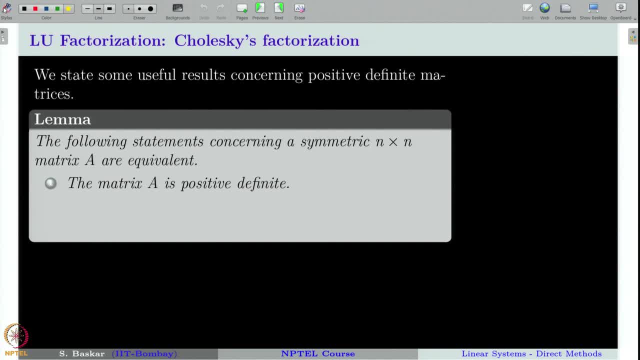 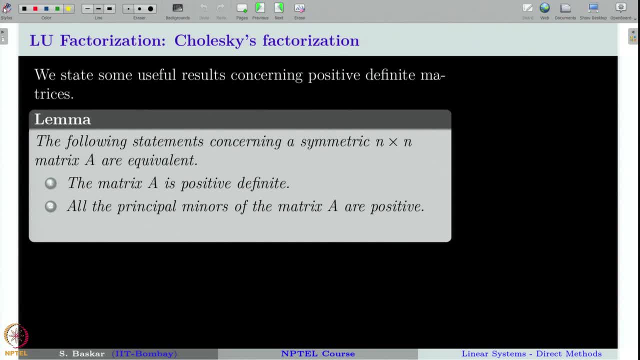 2 such. that is one equivalent condition for positive definiteness. You can see that principal minors can be computed relatively in an easy way. Therefore, this condition is more handy for us to check whether a symmetric matrix is positive, definite or not. Another equivalent. 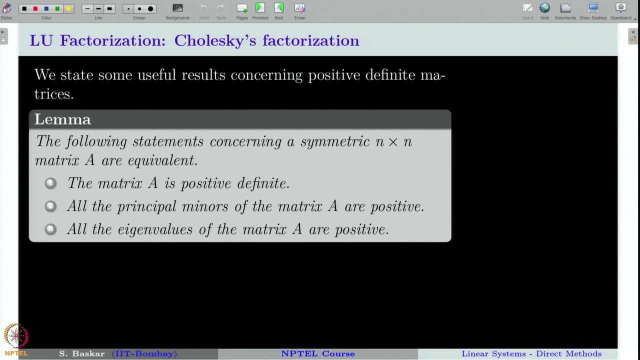 condition is that a symmetric matrix A is positive, definite if, and only if, all the eigenvalues of A are positive. Again, this can also be checked. well, finding Eigen values is little difficult computationally than finding principal minus. However, this can also be checked. We will not get into. 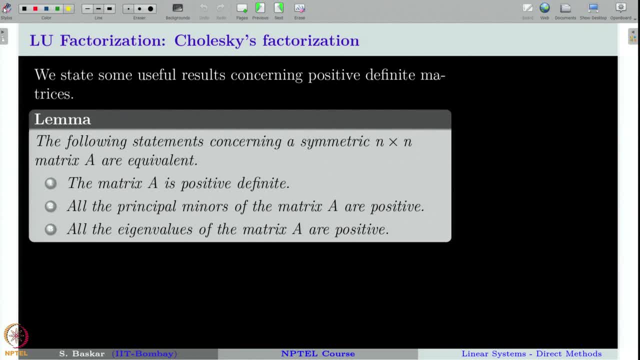 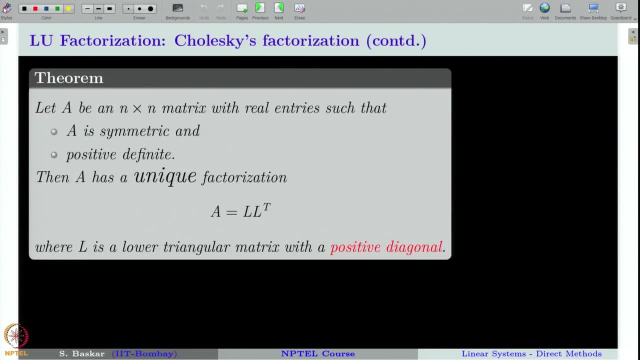 the proof of this lemma because it is a part of linear algebra course. but we will use these properties in our theorem on existence and uniqueness of Cholsky's factorization. The theorem says that: suppose you have an n cross n matrix with real entries. note that: 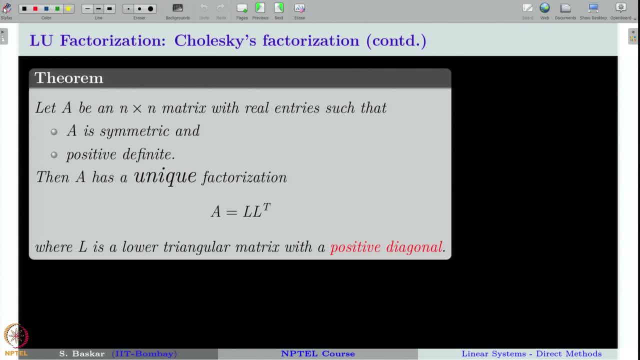 we will always work with matrices of real entries. Therefore, even if I do not tell this, you should keep in mind that we always work with matrices with real entries. So we have a matrix n cross n, such that it is a symmetric matrix and also it is positive. 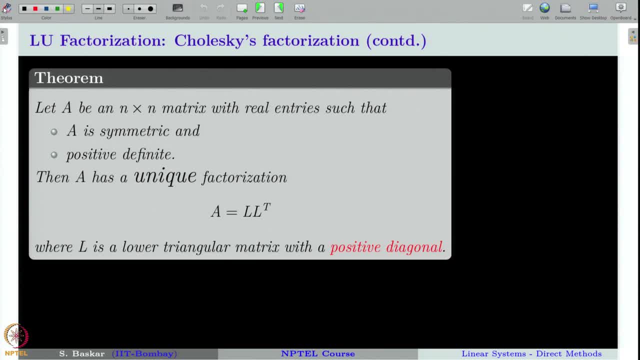 definite, Then we can always find the matrix n cross n. We can also find a lower triangular matrix, L, such that you can write A as L into L transpose. Moreover, if all the diagonal elements of this lower triangular matrix L are positive, then we can say that that is the only lower triangular matrix, such that A is equal to. 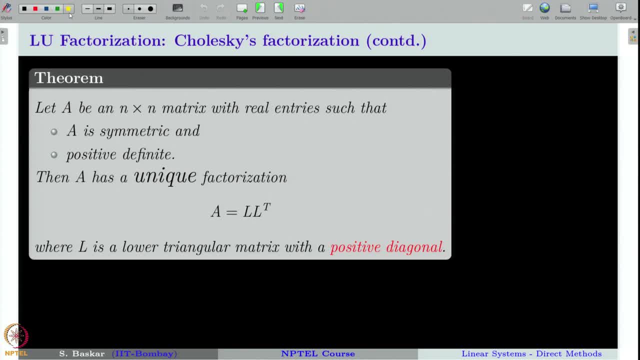 L into L transpose, That is, we get a unique. So when you say Cholsky's factorization, it means finding the lower triangular matrix L, such that A is equal to L, into L transpose. We are imposing this condition, that is, positive diagonal elements is just to make sure that. 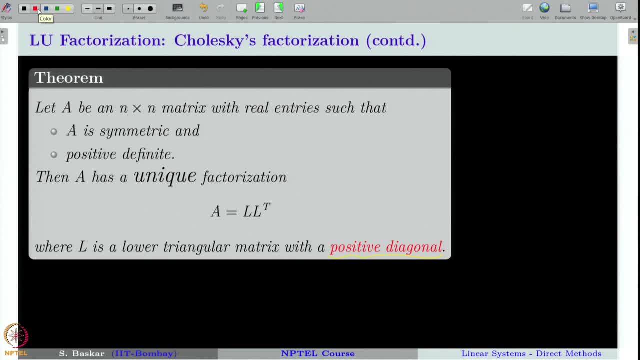 we have a unique way of obtaining the matrix L. In our computation you will see that all the diagonal elements of the matrix L will appear as L i i. square is equal to some number. Therefore, when you take square root, you get L i. i is equal to square root of that. 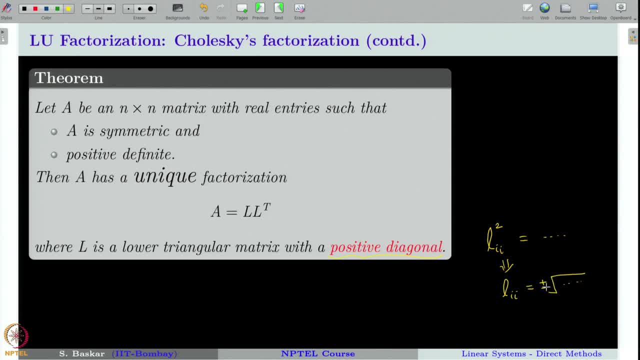 number. Therefore, you may have plus or minus also, So you have two choices here. to be very specific, We will always make our matrix Keep in mind that we will choose the positive sign for those diagonal elements. This is just to make the algorithm more precise, without any ambiguity of what sign we have. 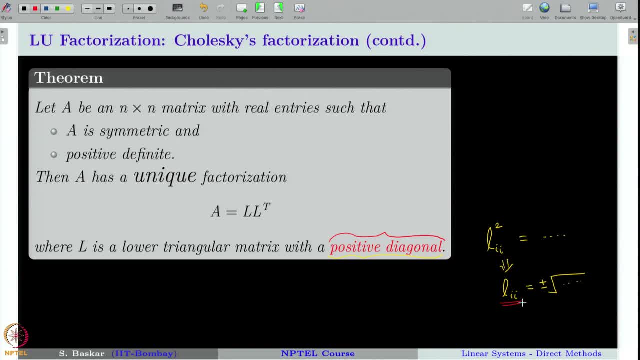 to choose. In that way, the theorem says that you will have a unique such matrix L. That is what the statement is. Let us try to prove this theorem. The proof is by induction. It means you first prove the theorem for the matrix A, which is a 1 cross 1 matrix. 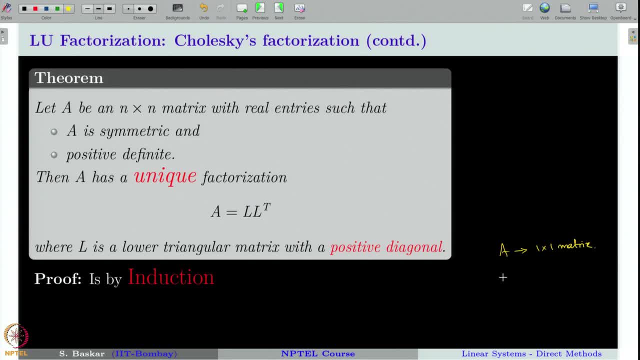 Then you assume that the factorization is possible for a k cross k matrix and then prove it for k plus 1 cross k plus 1 matrix. If you do so already, you have proved it is one 1 cross 1 matrix. 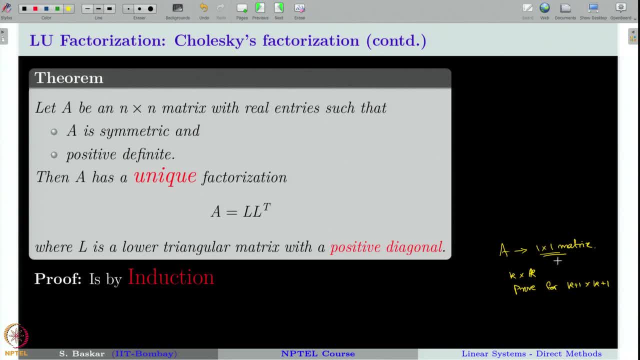 1 cross 1 matrix. Therefore it is true for 2 cross 2 matrix. Once it is true for 2 cross 2 matrix, then it is true for 3 cross 3 matrix, and so on. So that is the idea of induction. 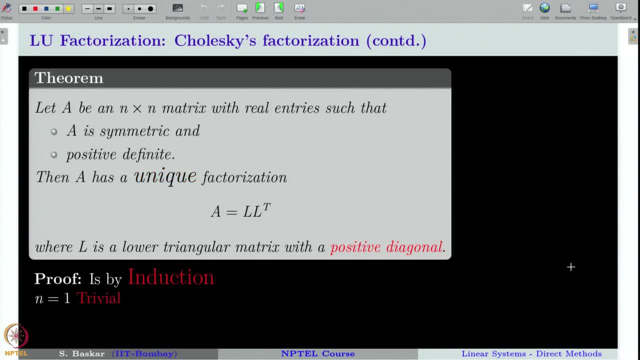 Therefore, the first step is to prove that a unique factorization is possible when A is a 1 cross- 1 matrix. Let us take A as A 1: 1.. Then obviously you can choose: L is equal to root A 1- 1.. Then you can see that A can be written as L into L. transpose, Of course. 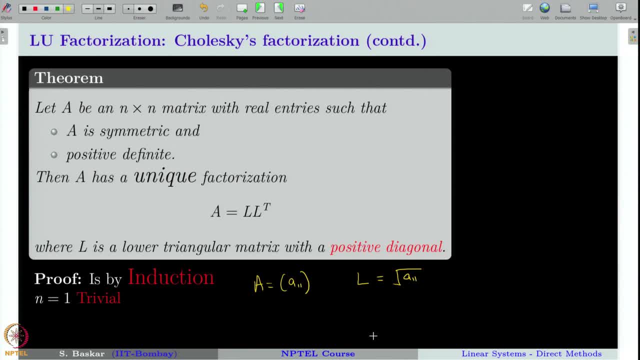 you can also choose minus root A 1- 1, but just because we made our mind to pick only the positive sign, we will not be able to do that. We will have plus root A 1- 1 here. Otherwise you can as well take minus. here There is. 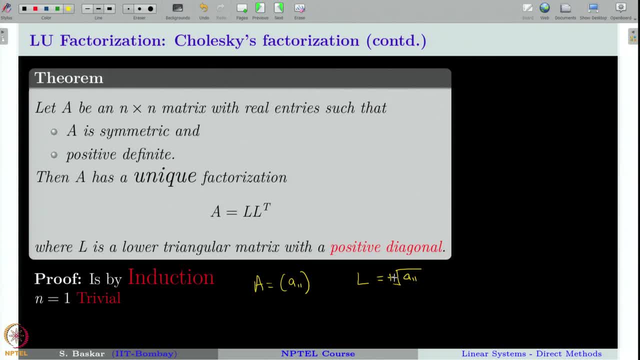 nothing wrong in that. Therefore the Chomsky's factorization is true. when the matrix A is a 1 cross, 1 positive definite matrix, It means A 1: 1 should be positive. That is how you are getting a real matrix L. Remember that L should be a lower triangular matrix with 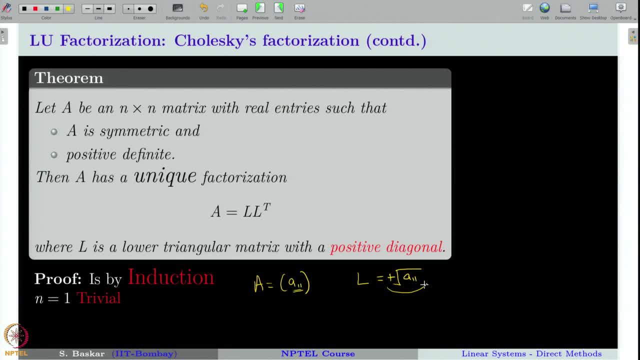 all its entries as real matrix L. Then only we will declare that Chomsky's factorization exists. Now we will fix our induction hypothesis As per that we will assume that the Chomsky's factorization holds for any K cross K matrix, for some natural number K. So we are taking a K, and then we 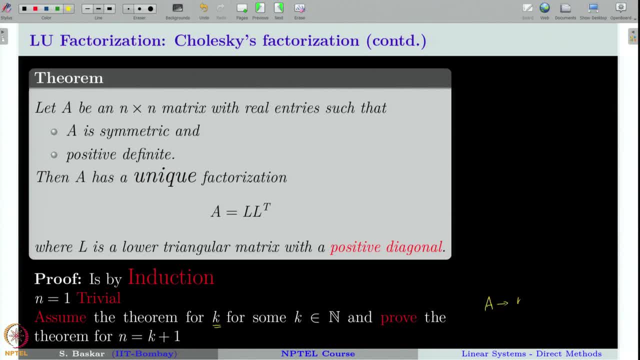 are assuming that if A happens to be a K cross K matrix, Then you can always find a L K such that A can be written as L K into L K. transpose Unique. such L K will exist with all its diagonal elements as positive. That is the assumption. 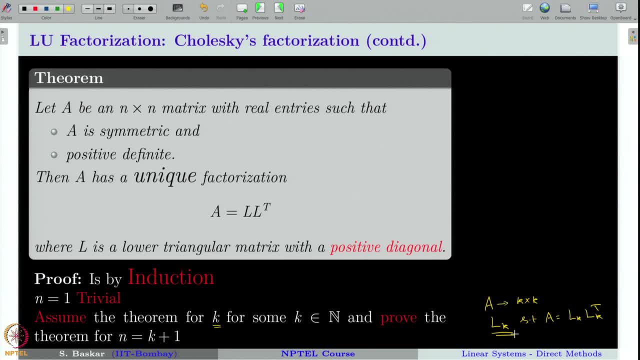 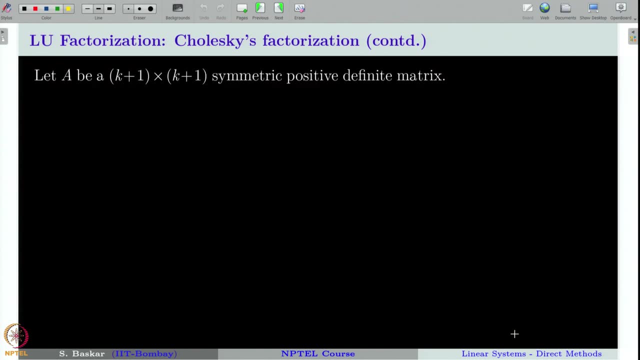 we are making, As per the induction method, what we have to prove? If we have a matrix which is K plus 1 cross K plus 1 matrix, then we have to prove that the Chomsky's factorization exists. So let us assume that A is a K plus. 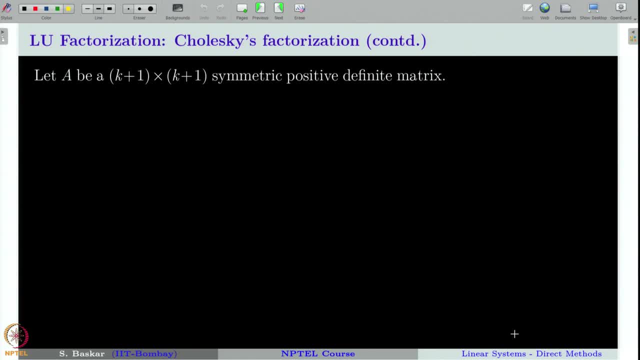 1 cross K plus 1 symmetric positive definite matrix. Now we have to find L such that A is equal to L into L transpose. Remember we have assumed that the Chomsky's factorization exists for any K cross K matrix. Then we have to prove that the Chomsky's factorization 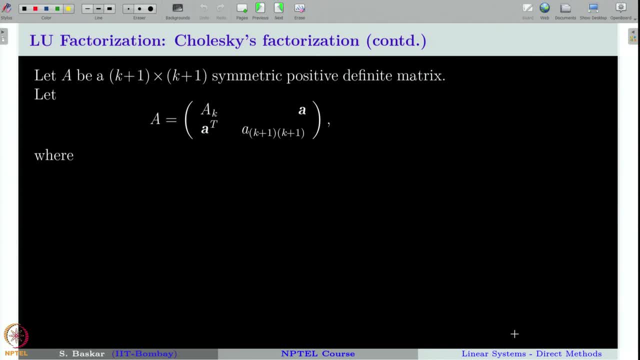 cross K matrix. Therefore, what we will do is we will write our matrix A as A K, which is the principal sub matrix of order K for A, and then we will write the remaining column vector as A and its transpose as A transpose, and then the last diagonal element, like this: 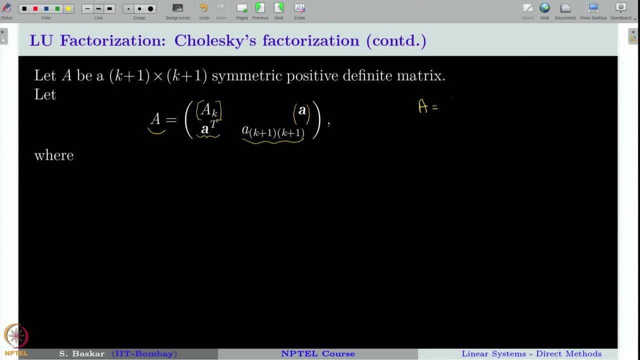 Just to visualize, let us take a 3 cross 3 matrix as A 1: 1, A 1: 2, A 1: 3, A 2: 1, A 2: 2, A 2: 3, A 3: 1, A 3: 2 and A 3: 3.. So here K plus 1 is equal to 3, we have taken in this. 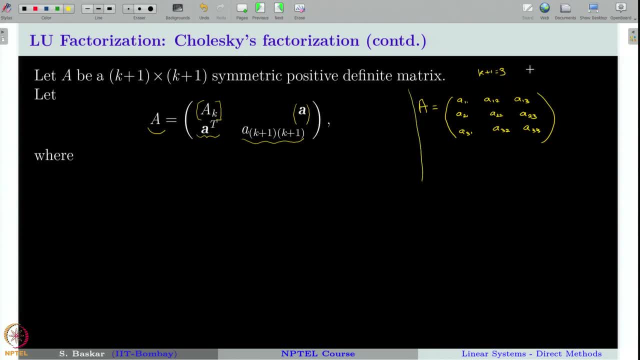 example. Therefore our K is 2.. So A K should be the principal sub matrix of A of order 2. It means it should be this matrix: this is your A 2 here. and then your column vector, small a, is taken as this: this is your A In all our. 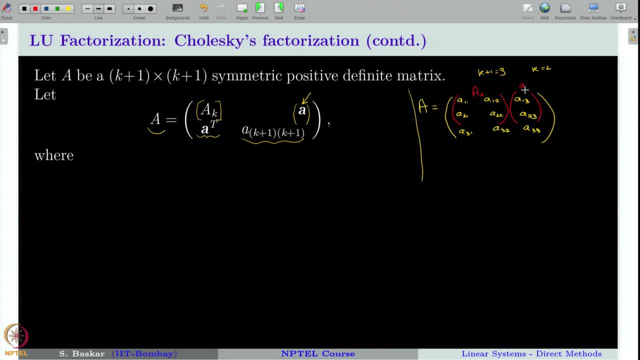 discussions in this chapter. we will always take a vector as a column vector. Therefore, its transpose, that is, the row vector, will always be written as A transpose. So this is what is A transpose. Remember, it is a symmetric matrix. Therefore, this and this- 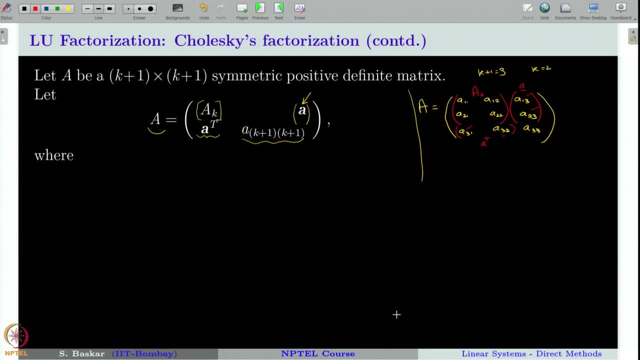 will be the same and this and this will be the same, That is, A 3- 1 will be equal to A 1- 3, and A 3- 2 is equal to A 2- 3, and then you have this element sitting here. So this: 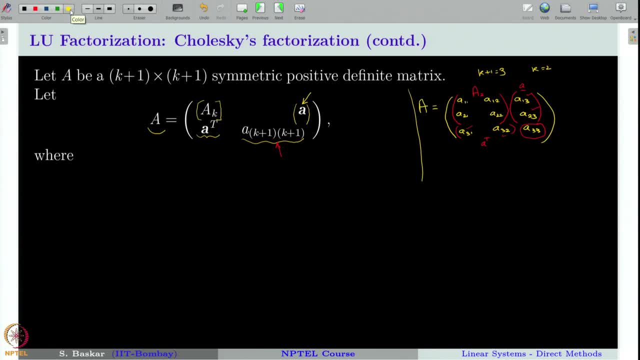 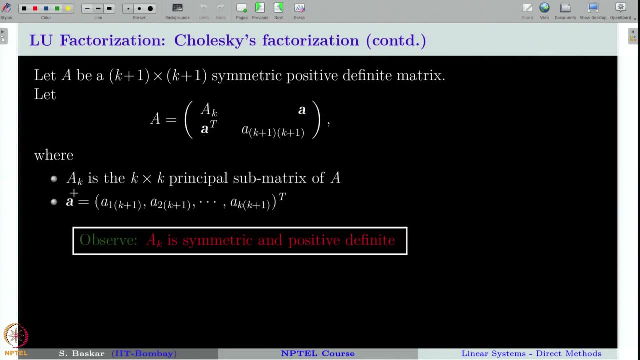 is how we are just splitting A into block wise, where A is the K cross, K, principal sub matrix of A and this vector, A, is the column vector At the last column, removing the diagonal element. that is A, K plus 1, A K plus 1.. You can observe: 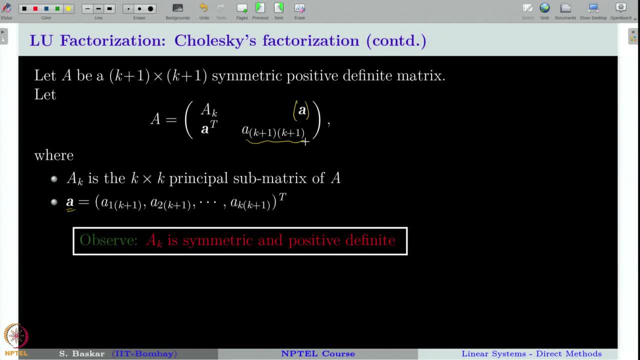 that A is a symmetric matrix. Therefore, A K is also a symmetric matrix. Also, you can see that A- K is a positive definite matrix. because A is positive, definite by our lemma, all its principal minus are positive. In particular, the matrix A is a positive definite matrix. 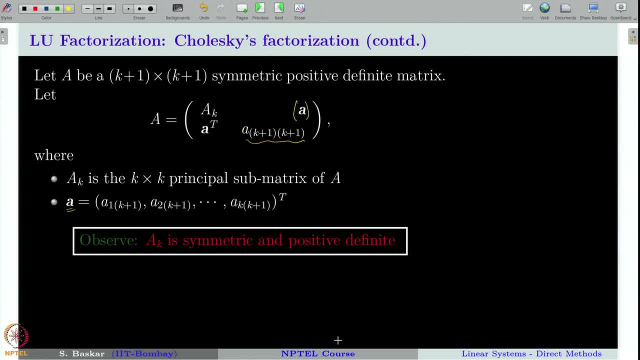 The principal minus of A, K are also principal minus of A with lower order. Therefore they all are also positive in turn. A K is also a positive definite matrix. This is an observation. Therefore, by our induction hypothesis you can find the Cholskis factorization for A. 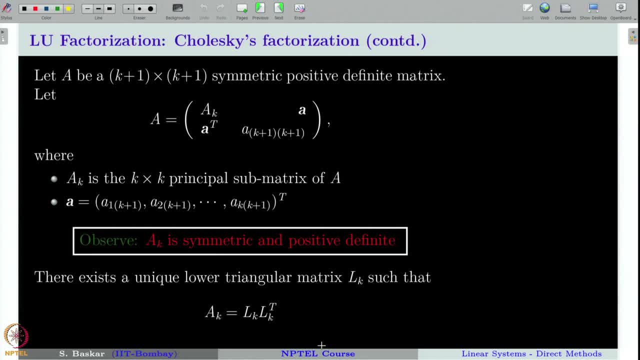 K, find a unique lower triangular matrix, Lk, such that Ak equal to Lk into Lk transpose where all the diagonal elements of Lk are positive. This is the assumption as per our induction hypothesis. Now let us see how to construct the Cholesky's factorization for A with the help of the Cholesky's 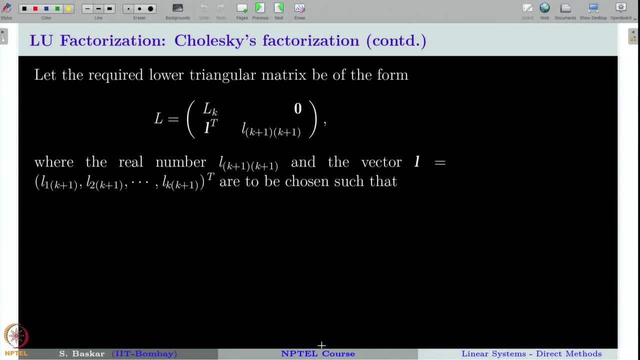 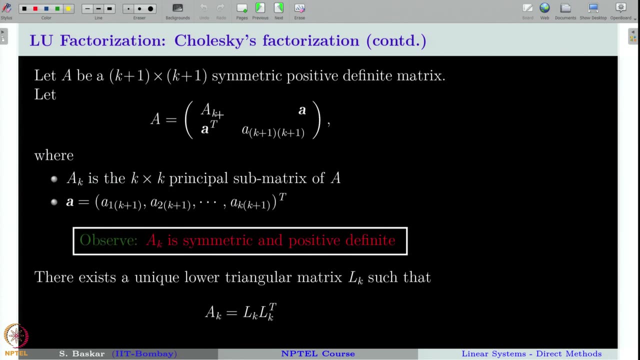 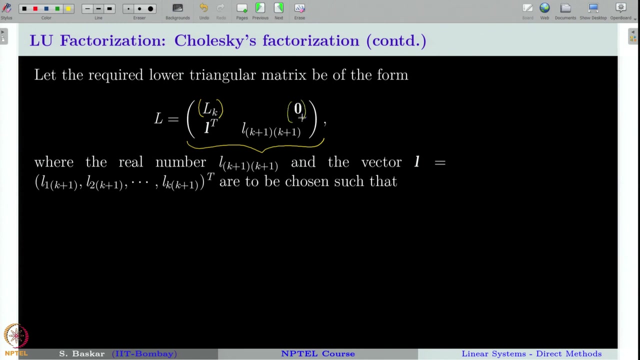 factorization of Ak. Let us propose that the Cholesky's factorization of A looks like this matrix, where Lk is coming from our Cholesky's factorization of Ak, and then all these elements are 0, because it is a lower triangular matrix and you have a vector L. 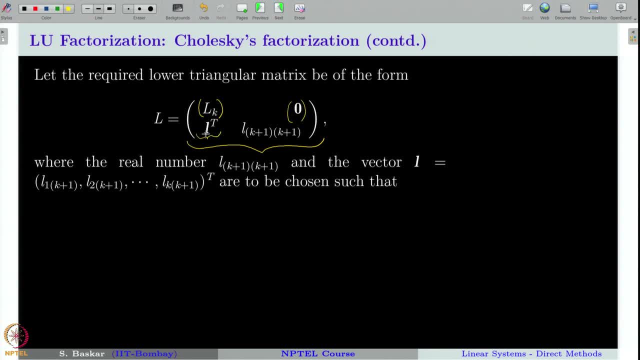 The vector L, which is written in the row form. therefore it is L transpose. and then this is a number: Lk plus 1, k plus 1.. Now here we know this. this is known to us as per our induction hypothesis. Therefore, we do not need to compute that, but we need to compute. 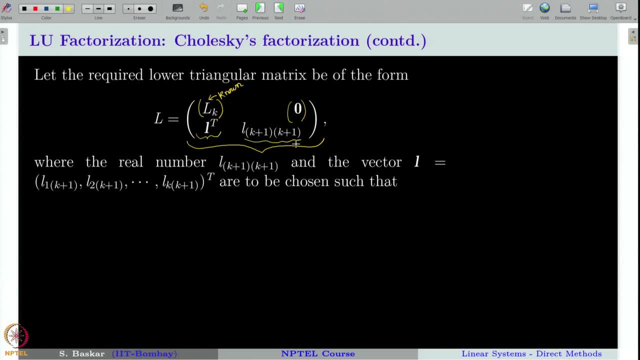 the vector L and the real number Lk plus 1, k plus 1.. Now how we have to find that we should find these quantities in such a way that a is equal to L into L transpose. so that is our Cholesky's factorization. So have to find this vector. 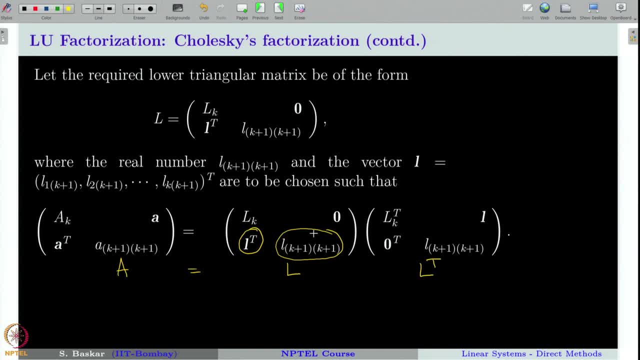 and this real number. How are we going to find this? Let us see. well, what we can do is You: take this, the first block of the matrix L- this is the row block- and multiply it with the last column of L- transpose. that will give you L. k into L is equal to. we have to. 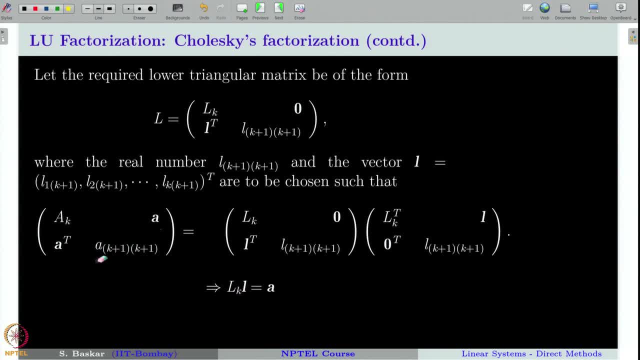 compare that with the corresponding entries of the left hand side matrix, which happens to be the vector A. So the vector A is known to us and therefore we got a lower triangular system with solution as the unknown vector L. Now how will you find it? Well, you can. 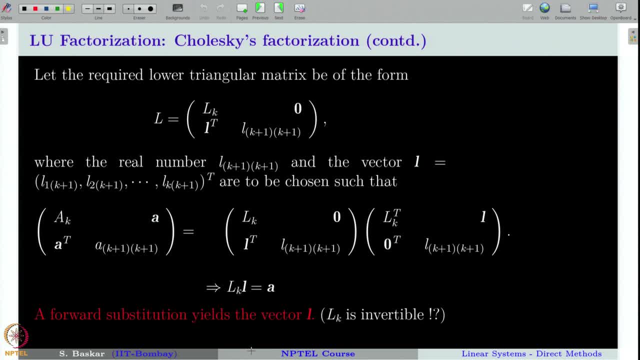 just use the forward substitution To get the vector L. because L k is a lower triangular matrix, you do not need to go for any elimination process. You can simply use the forward substitution to get the vector L, provided the matrix L k is invertible. How do we know that the matrix L k is invertible? 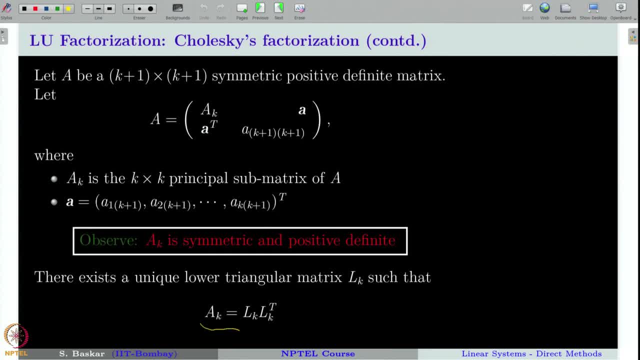 Well, you can see that from the way we have constructed L k. We have constructed L k such that A k equal to L k into L k. transpose. Now you take the determinant on both sides, you have A k. determinant is equal to determinant of L k square. but 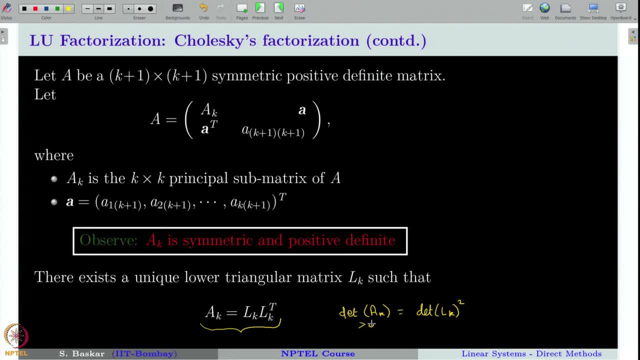 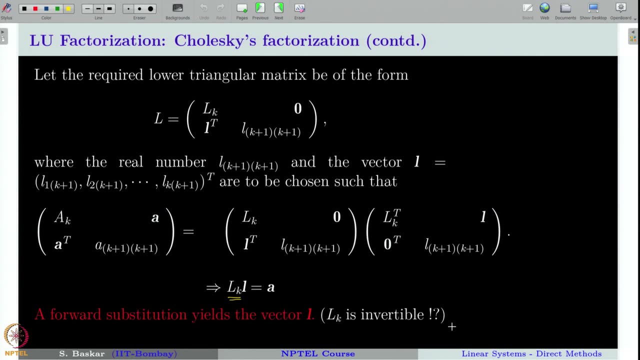 this is positive because A is a positive definite matrix. Therefore, this is surely non-zero. that is what we can see From the way L k was computed. L k is an invertible matrix, So you will get a unique vector, L. 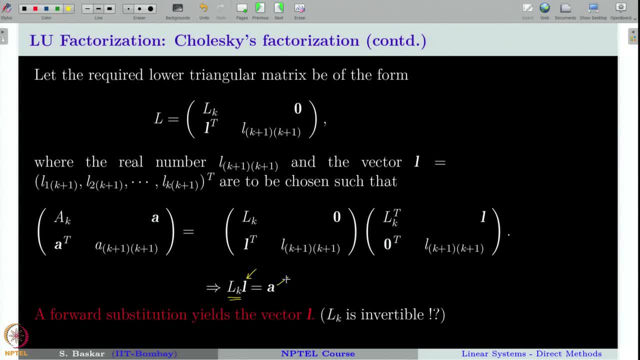 such that L, k, L is equal to A, which is a known quantity. So we obtained this vector L. Now we need to only find this real number. that is the only part left out for us. Let us see how to find it. 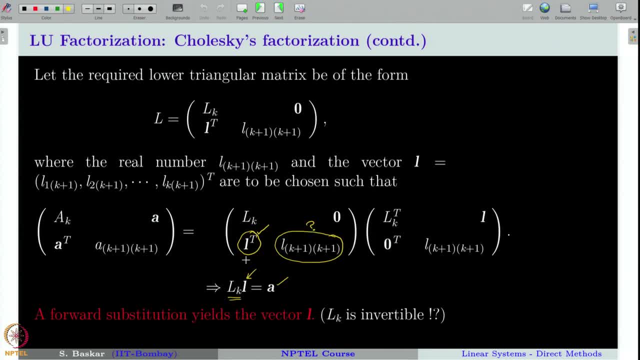 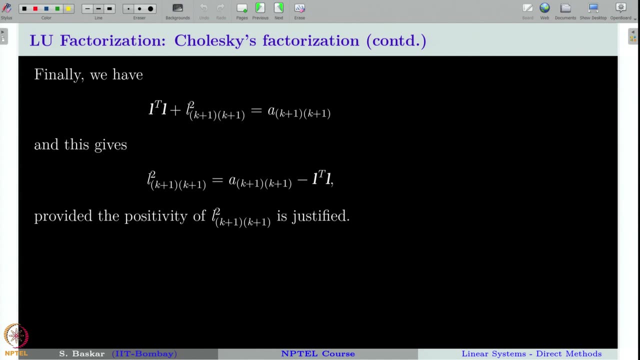 Again, what we will do is you take the last row of L and multiply it with the last column of L transpose. That gives us the vector L transpose into L plus L, k plus 1, k plus 1 square. That needs to be compared with the corresponding element of the matrix A and 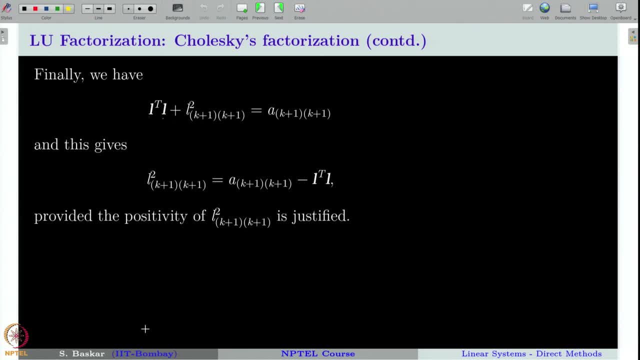 that is going to be A k plus 1, k plus 1.. Now that gives us L square k plus 1. k plus 1 is equal to A k plus 1 k plus 1 minus L. transpose L Now from here you may take L k plus 1. k plus 1 is equal to root: A k plus 1 k plus 1 minus. 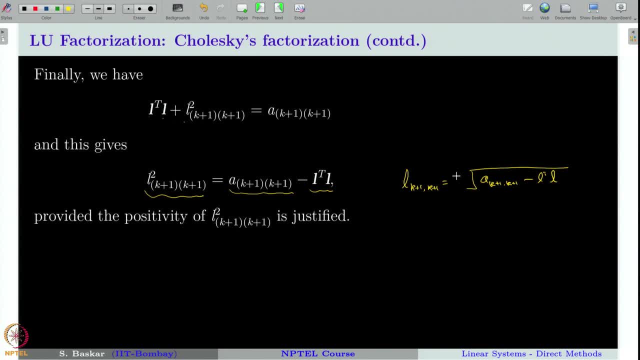 L transpose into L. Of course you have to have plus or minus, but we have already made our mind that we will take only the positive sign. Therefore, I will take here only positive sign. but then the question is: is this real? In other words, we have to first justify that. 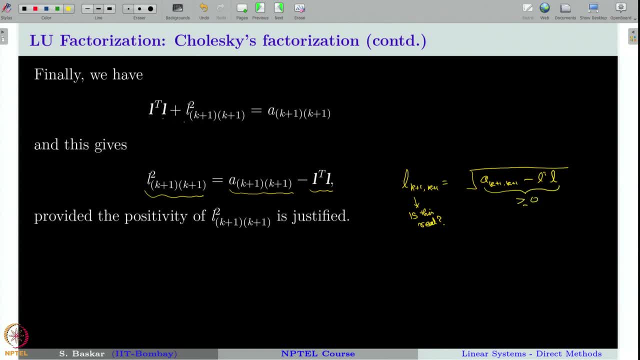 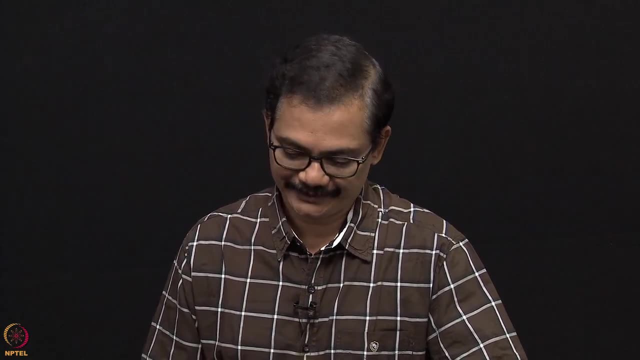 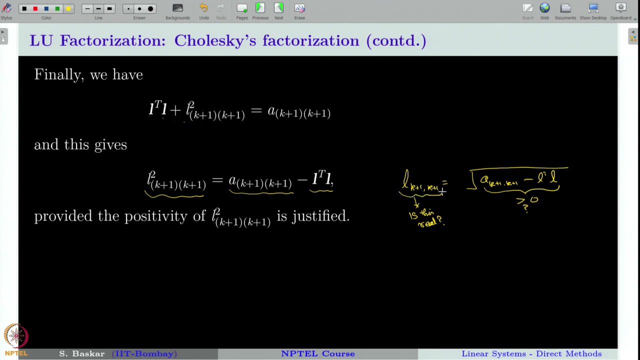 is this greater than 0?? That is the question because, remember, in order to say that the Cholesky factorization exists, we have to find a lower triangular matrix with all its entries as real numbers. Therefore, this number should also be a real number, but it need. 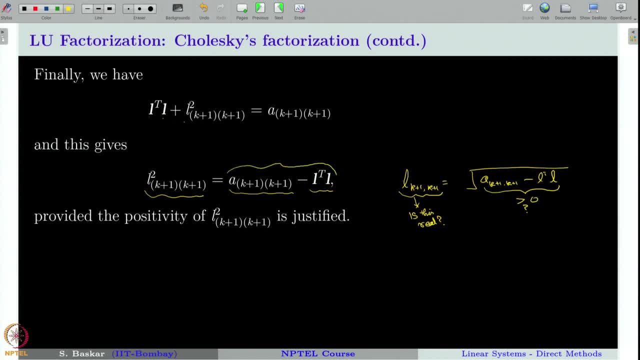 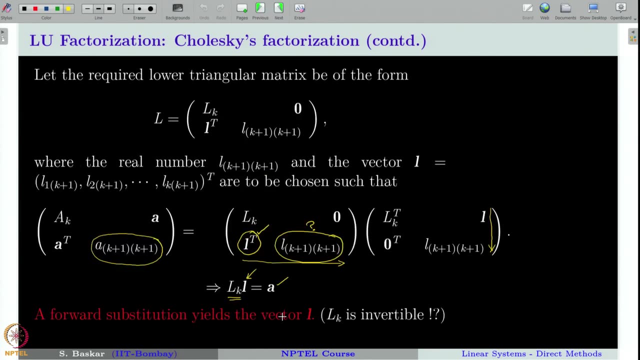 not be, because if this number happens to be negative, then it is not a real number. You will have L? k plus 1, k plus 1 as an imaginary number. Therefore, you have to justify this. How will you justify it? Again, go back to the form that we are writing. You take determinant. 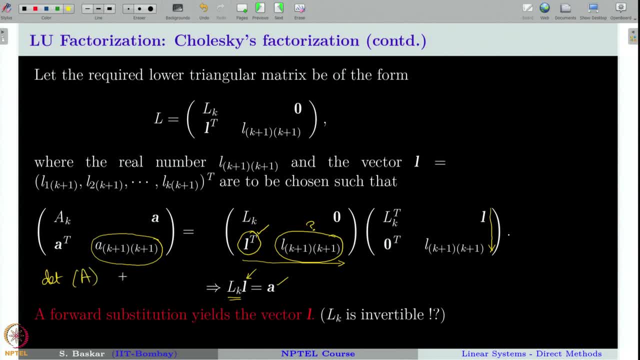 of A, and that is equal to determinant of L, into determinant of L transpose, Which is nothing but L square. What is determinant of L, Determinant of L is determinant of L k, into L k plus 1, k plus 1.. That square means this is square, and square Now determinant. 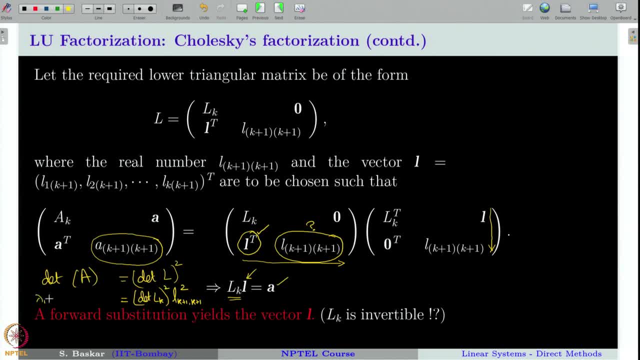 of A is nothing but the product of all its eigenvalues. Therefore, you can say that the product of all the Eigen values of A is equal to. this is a positive number because we already know that L k exists. it means all its entries are real. that is already assumed, Therefore. 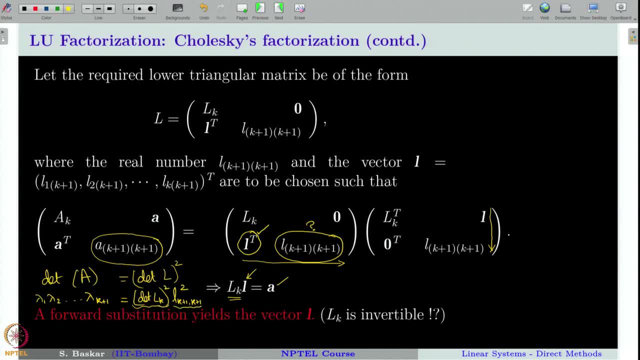 this is a positive number, and this is what we do not know, whether it is positive or not. Now you can see that all the Eigen values of A are positive. why? because A is a positive definite matrix. So we have stated one equivalent property of positive definite matrix in the 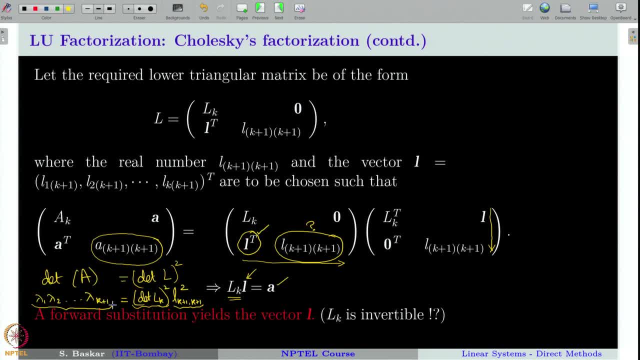 last lemma that all its Eigen values are positive. Therefore the left hand side is the product of positive numbers. therefore it is positive. That shows that. So L? k plus 1 k plus 1 square is a positive number. Remember, just because you are squaring, 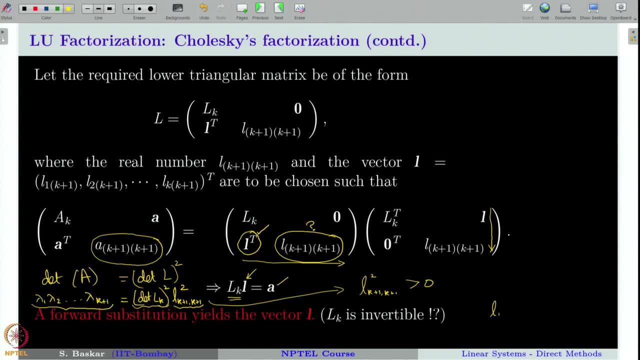 this does not mean it is positive. Say, for instance: if L k plus 1, k plus 1 is equal to i, then its square is minus 1.. Therefore you just cannot directly say that this is a positive number. you have to justify this. 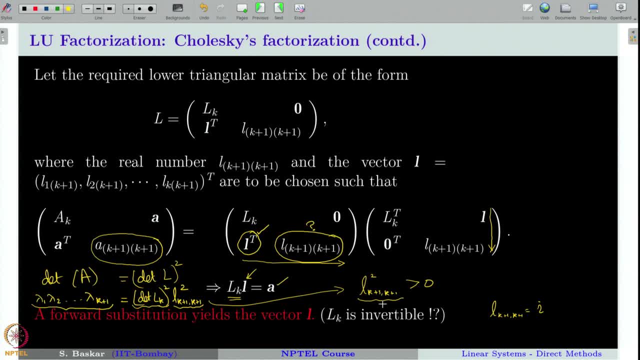 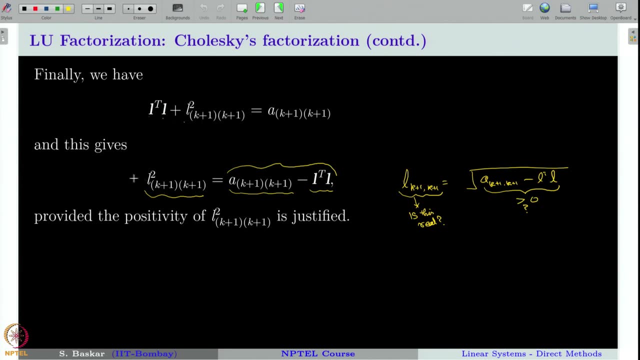 This is because we have not yet proved the existence of Cholsky's factorization. In fact, that is what we are trying to justify: that this is positive and that comes from this representation. Therefore, we have proved that this is positive and that implies that 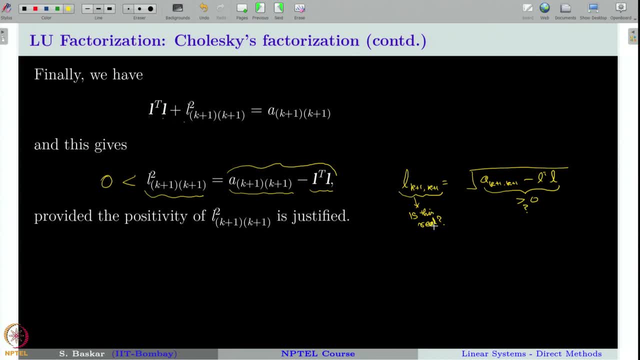 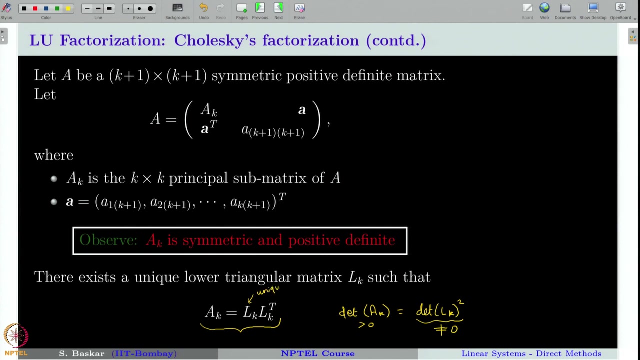 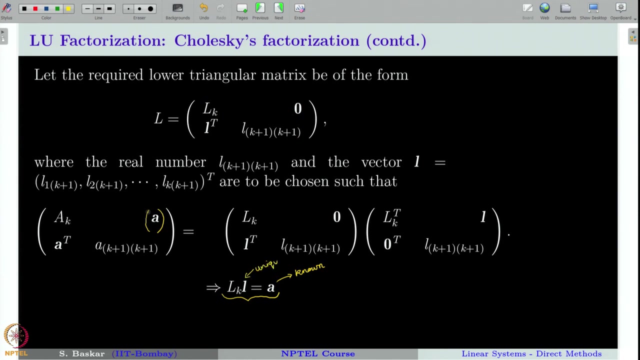 L, k plus 1. k plus 1 is a real number and that proves the Cholsky's factorization existence. And also you can see the way we have constructed that the Cholsky's factorization is unique. Why? Because from the induction hypothesis L k is unique. This system has a unique solution. 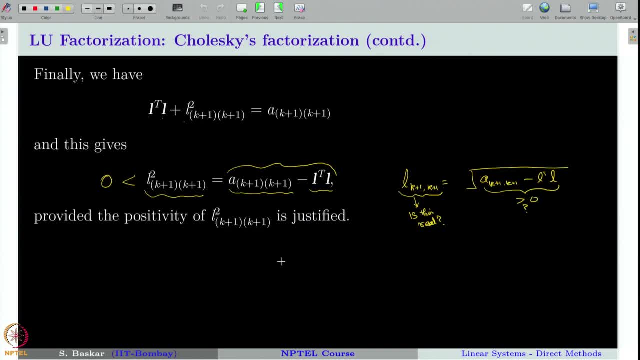 L. Similarly, this also is a unique representation. Therefore, with all this, we can see that our Cholesky factorization is unique, provided that all the diagonal elements sign or fixed as a unique sign. either it should be positive or negative. You can see that at every stage. 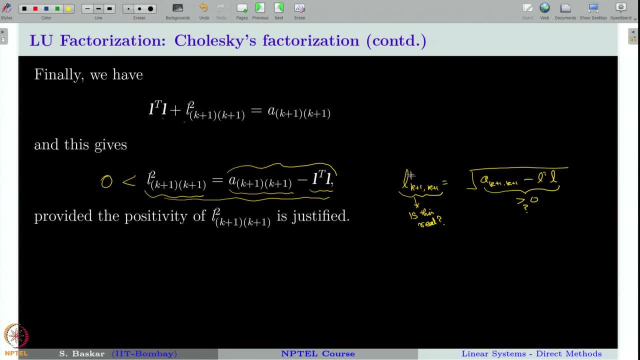 of induction, you are taking the square root for getting the diagonal element. There you have two choices: you may go for a plus sign or minus sign. So we made our mind to take only the plus sign in all the steps. In that way we have a unique factorization that you 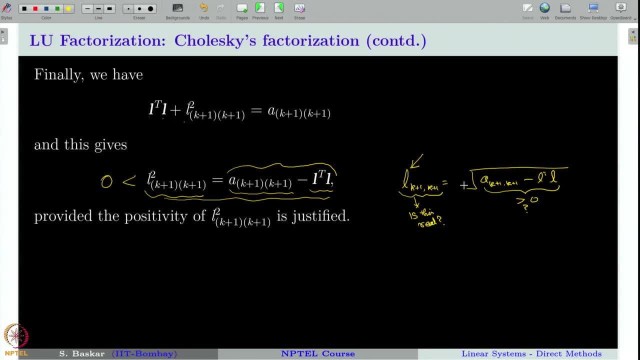 have to keep in mind. There is nothing wrong in taking minus in all the steps. also, that gives a different Cholesky factorization. So as such, Cholesky factorization is not unique, but if you fixed the diagonal elements sign, then it is unique. Let us take an example. Let us take the matrix. 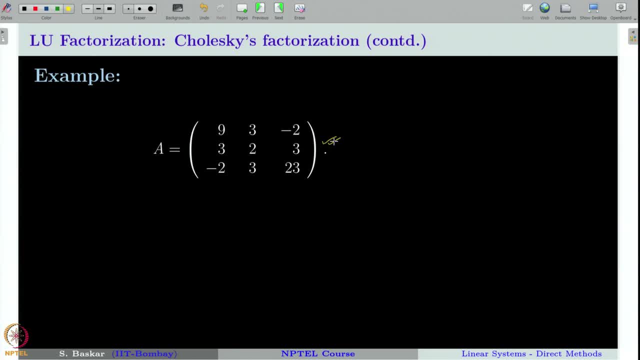 A as given. like this, You can observe directly that it is a symmetric matrix. also, you can see that it is positive definite. How will you do that? One easy way out is to check all its principal minors are positive. The principal minor of order 1 is 9 for this matrix. 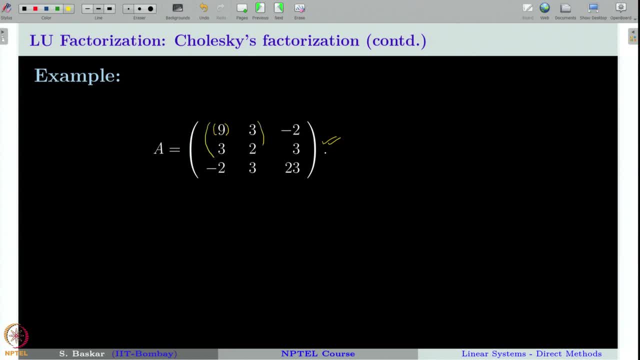 that is positive. The principal minor of order 2 is 9 into 2 minus 9, that is again 9, right? that is also positive. and you can also see the determinant of A is positive. Therefore this is a symmetric and positive definite matrix. Therefore we can find a unique Cholesky's. 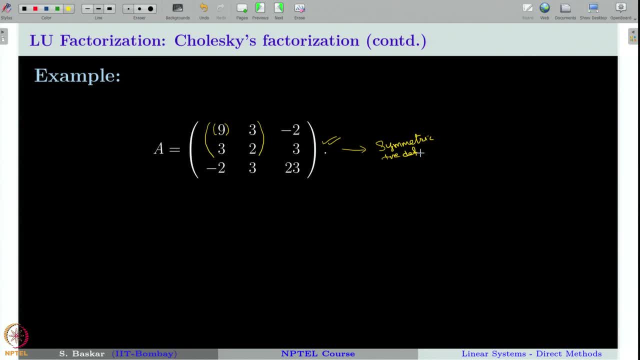 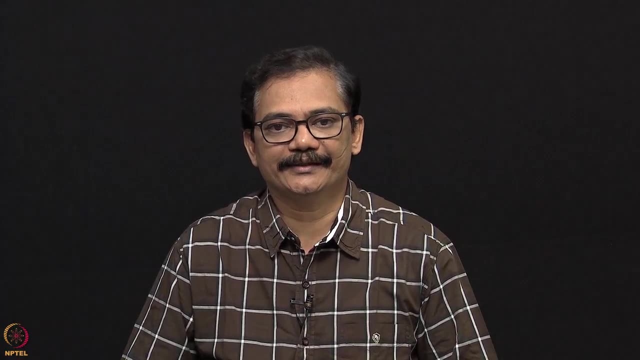 factorization with all the diagonal elements being positive. Let us see how to compute that. There are many ways to compute, but we will just follow the construction procedure we have done- We adopted in the previous theorems- proof- and try to construct the Cholesky's factorization. 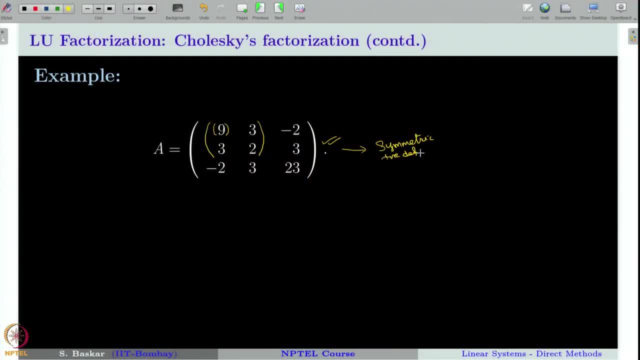 for this matrix. For that we have to first compute L1.. What is A1? A1 is nothing but 9. Therefore L1 can be taken as 3 or minus 3.. Again, I am emphasizing: we will always. 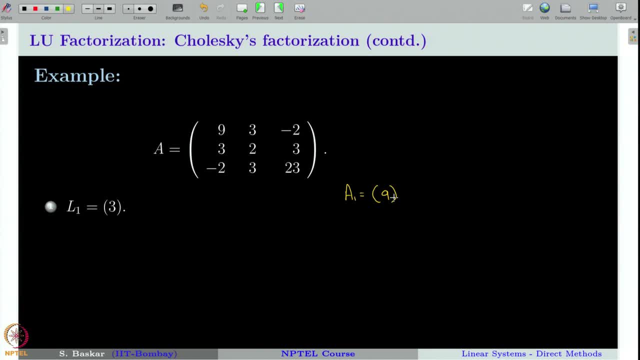 take the positive sign. Therefore we are taking L1 as 3.. So with that we will go to find what is L2.. For that we will write L2 as L1 0 and then L2 1, L2 2. right, L1 is 3.. Therefore it is 3: 0, L2 1. 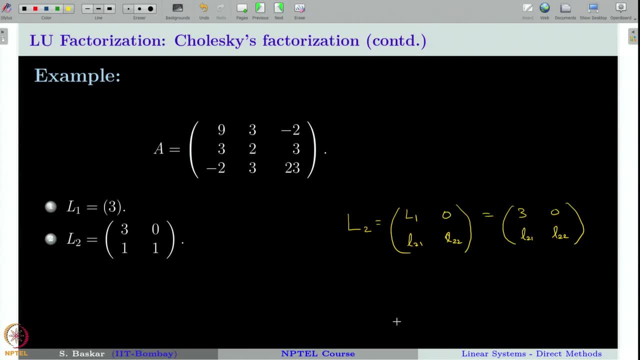 L2 2.. Therefore it is 3 0 L2 1, L2 2.. Therefore, it is 3 0 L2 1, L2 2.. Therefore, it is 3 0 L2, 1 L2 1, L2 2.. We have to find what is L2 1 and L2 2, such that A2, which is nothing but. 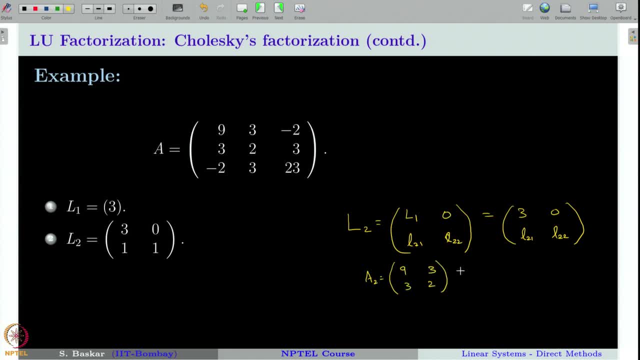 9 3 3 2. equal to 3: 0 L2 1. L2 2 into 3 L2 1 0 L2 2 and that is going to be equal to 3 times L2 1.. 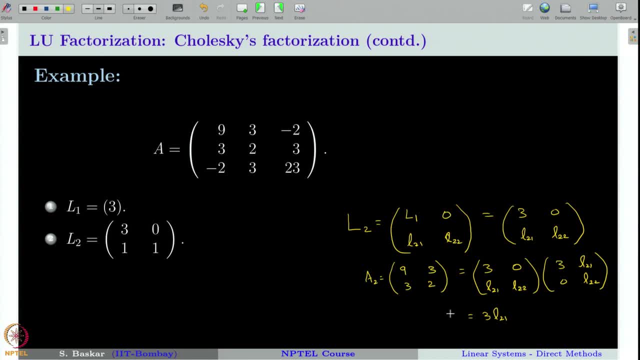 1 is equal to 3, that implies L 2: 1 is equal to 1.. Similarly, L 2: 1 square plus L 2: 2 square is equal to 2. that will again imply that this is going to be L 2: 2 square equal to 1 or. 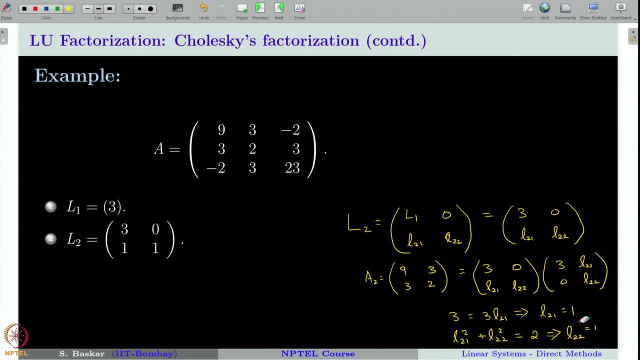 L 2, 2 is equal to 1.. Again, remember, whenever there is a diagonal element, we will always get it in terms of the square of that element and then, when you take the square root, we will always take the positive sign and that gives us L 2 as 3, 0, 1, 1.. 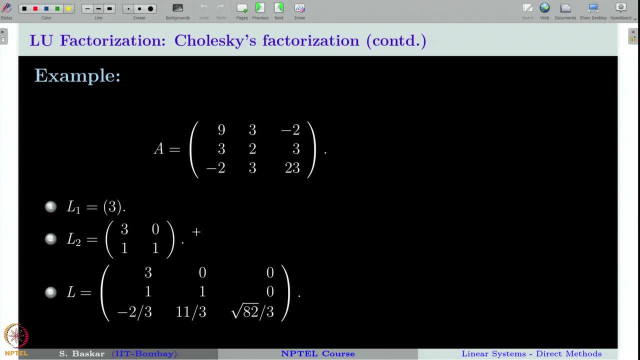 Let us now compute L 3, which is also the required Cholsky's factorization. For that, we will take L as L 2, and then L transpose L 3, 3, and then this is a 0 vector. That gives us: 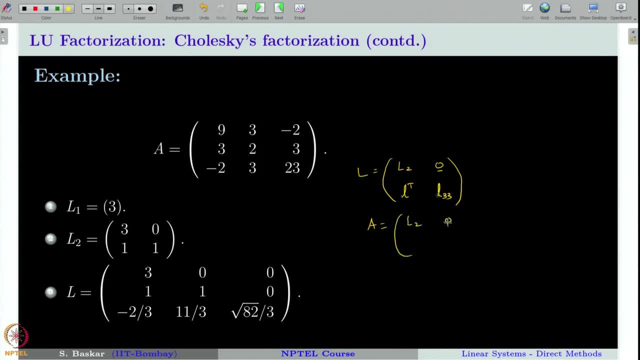 A is equal to L 2, 0. L transpose L 3, 3 and then its transpose, that is, L 2 transpose, L 0 transpose and L 3: 3.. When you take the first block row with the last column, here we get L 2. L is equal to. 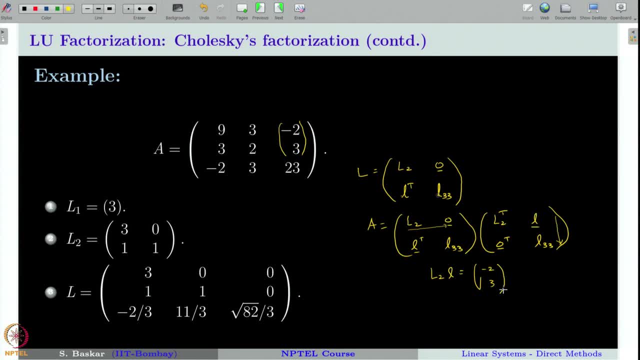 this vector minus 2: 3, that gives us L 3: 1.. So remember, this is L 3: 1, L 3: 2 and L 3: 3.. L 3: 1 is equal to L 2. L transpose L 3: 2 and L 3: 3.. 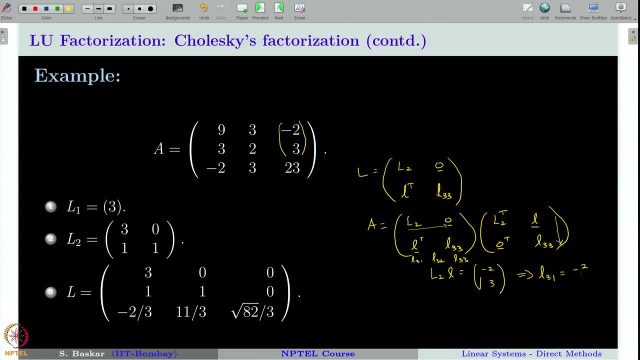 L 3: 1 is equal to L 2, L. transpose L 3: 2 and L 3: 3.. L 3: 1 is equal to minus 2 by 3 and L 3: 2 equal to 11 by 3.. So that is what we have. 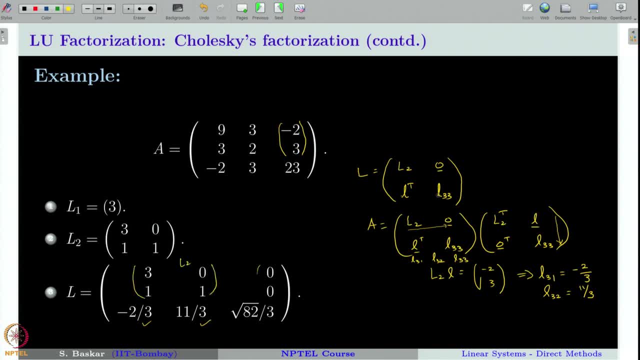 here. This is our L 2 and this is the 0 vector, and we have L transpose here. Now we have to find the diagonal element L 3, 3.. For that we will multiply this with L transpose- L 3 plus L 3, 3- and multiply this with the last column of L transpose. That gives us L transpose. 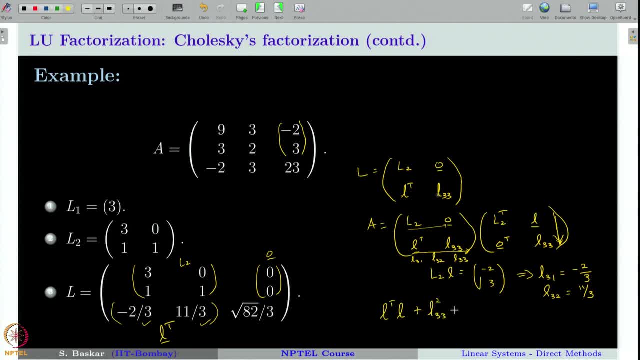 L plus L 3, 3 square is equal to 23.. That gives us L 3, 3 square equal to 23 minus 4 by 9 plus 121 by 9.. And that 9 into 23 minus this is going to be 8.. 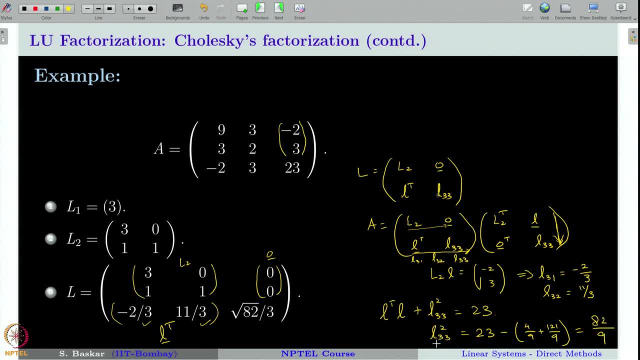 9 into 23 minus this is going to be 8.. So 9 into 23 minus this is going to be 8.. So 82 by 9.. And therefore, if you take the square root on both sides and choose the positive, 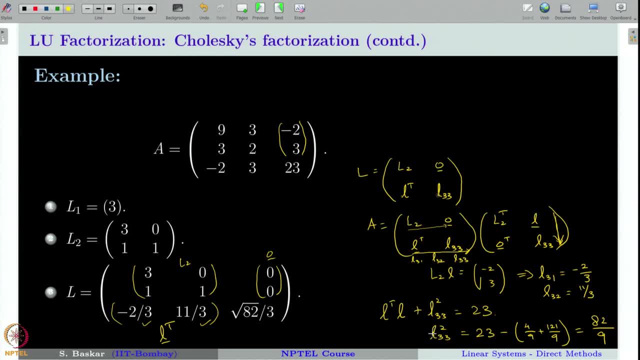 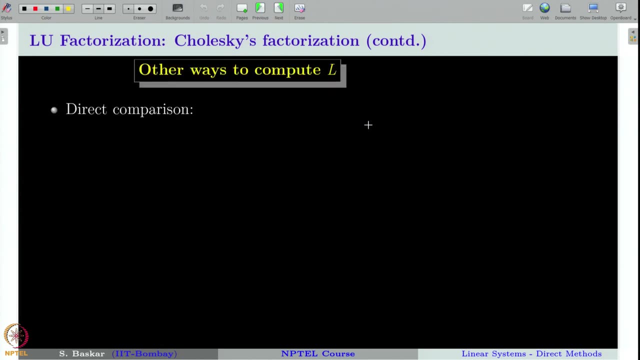 sign we will have L 3: 3 equal to root 82 by 9.. And that gives us the Cholsky's factorization for the matrix A. given like this, This is not the only way to compute Cholsky's factorization. 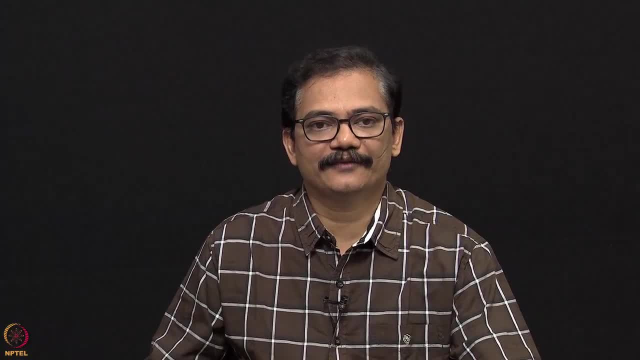 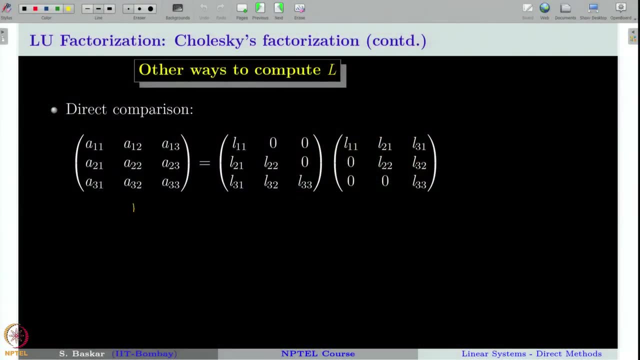 Recall, in the Doolittle case. we computed the Doolittle factorization by direct comparison. What we did? We wrote A is equal to L into L. transpose, Of course, in Doolittle all the diagonal elements of L are 1. So you have to write such an L and then find the other. 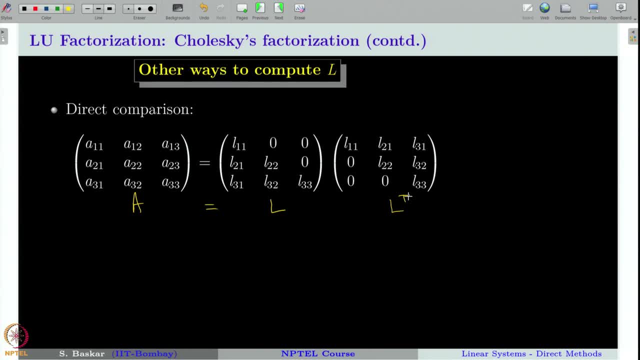 entries of L as well as U. So in fact this was u there in the Doolittle factorization, but here in Cholsky's factorization we have to take it as L transpose itself Now, just like how we did with Doolittle factorization. what? 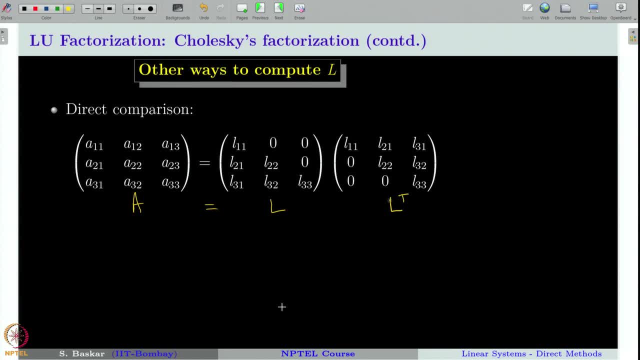 we did the right hand side product of two matrices. we just multiplied them and then compared the elements of the right hand side matrix with the corresponding elements of the left hand side matrix and we got all the elements of L and U there. The same idea can. 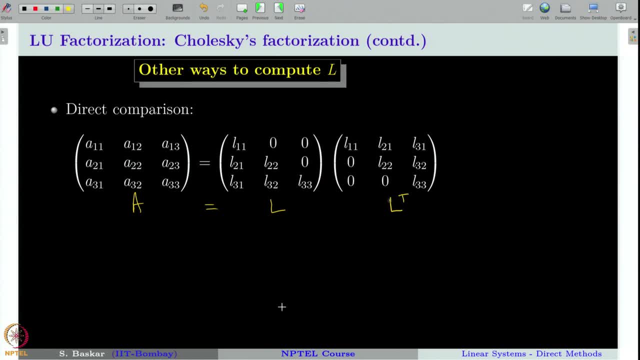 be followed in constructing Cholsky's factorization. also, you need not go step by step as we did in the last computation. This is to make the proof of the theorem more rigorous. we used it in the form of an induction. Otherwise you can also go for a direct comparison calculation. 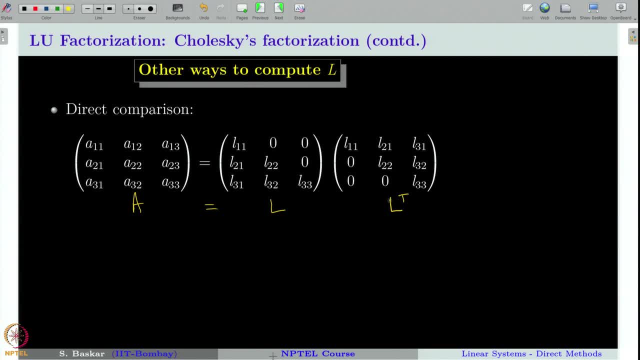 which we have done. So this will also lead to a very efficient algorithm. Let us see how these expressions look like. Well, L 1- 1 can be directly obtained as root: a 1, 1. remember again, we are fixing our sign as plus. that is why we got it. otherwise, you can also take minus root: a 1, 1.. Now L. 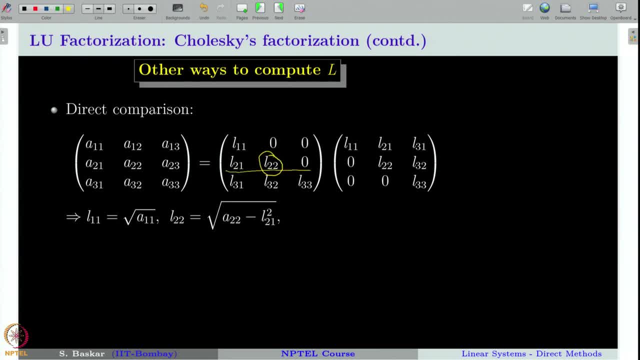 2: 2 is obtained by multiplying this row of L with this column of L transpose, and that gives L 2: 2 as this. Similarly, to get L 3: 3, you can multiply this with this and that gives you L 3- 3.. All. 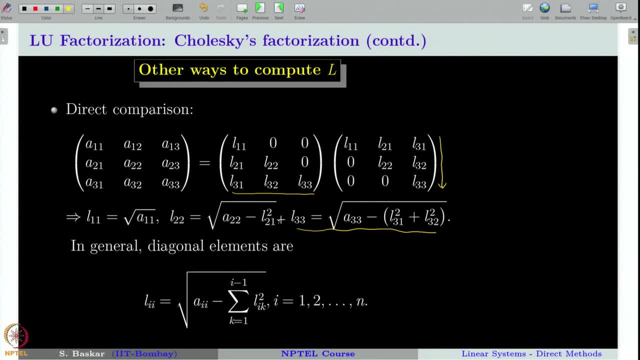 the diagonal elements are therefore obtained In general. if your matrix is a n cross n matrix, you can just look at these expressions and try to generalize how this expression will look like for a n cross n matrix that will be given as L i. 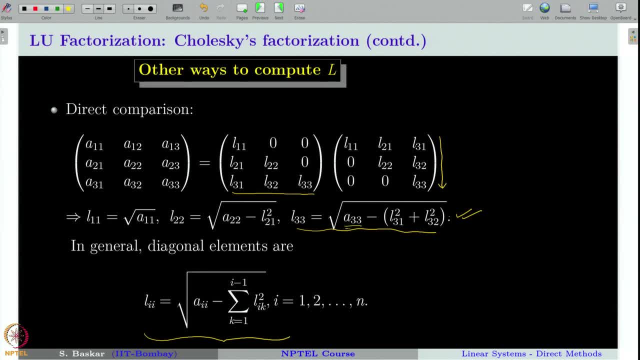 L, i, i is equal to root a i, i minus you have the sum starting from k is equal to 1 and goes up to i minus 1.. So here it is 3, therefore it goes up to 2.. Similarly, if you are computing, 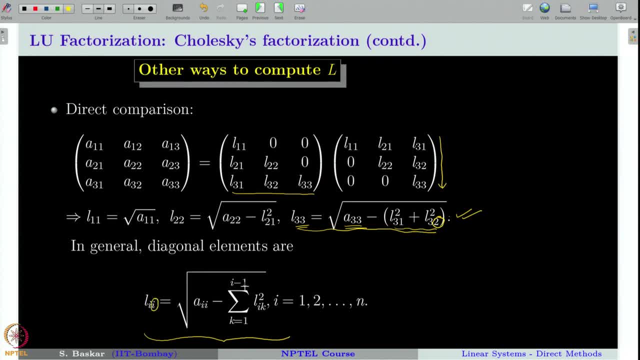 the diagonal element at the ith row, it goes up to i minus 1, because i is already there. that is what you are computing: i plus 1. onwards, the entries are 0 because it is a lower triangular matrix. Therefore, this will go only up to i minus 1.. 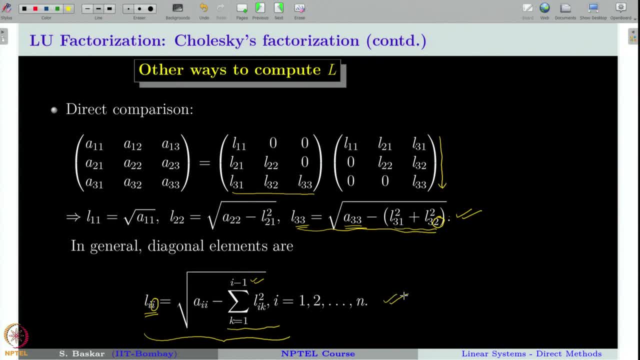 So, therefore, the diagonal elements are given by this expression, how the non diagonal elements are obtained. again, let us see to get this element. you can just multiply this row with the first column of L, transpose, and that gives you L: 2, 1, i, 3.. So that is n cross, n x, m, square, V x 1.. So that gives L 2, 1.. theownik div. you can add the diagonal elements i, or that will be 1, then기를 to the othernet of V, 1 equal to 0.. 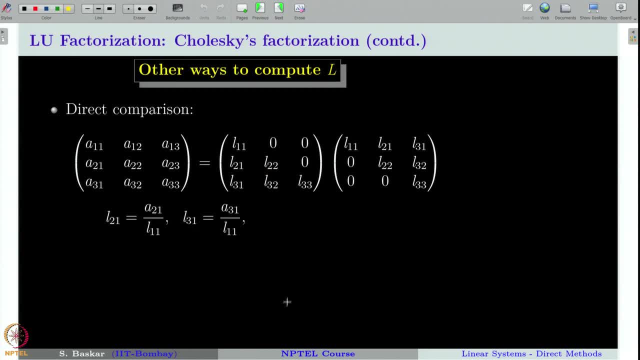 L 3: 1 we have to find for that. you take this and again you do multiplication with the first column of L, transpose. that gives you L 3, 1. and how will you get L 3, 2? Well, you multiply this with the second column and that gives you L 3, 2 again. you can just observe the expression. 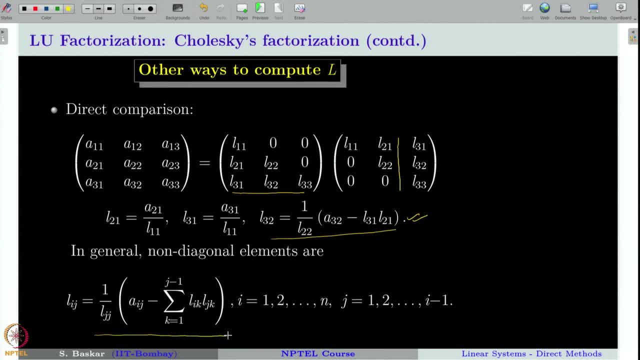 and try to generalize it: for any n, cross, n, symmetric, positive, definite matrix A, and that gives you this expression. Remember this has to go for each column other than the diagonal element. all the elements after diagonal elements are also not computed. Therefore, j should go from 1, 2 up to i minus 1, and this has to be done for all the rows, right, therefore?